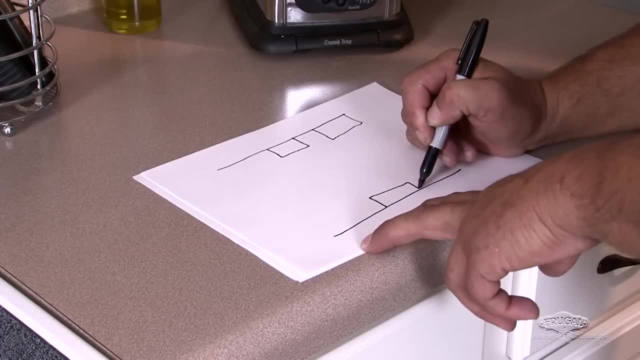 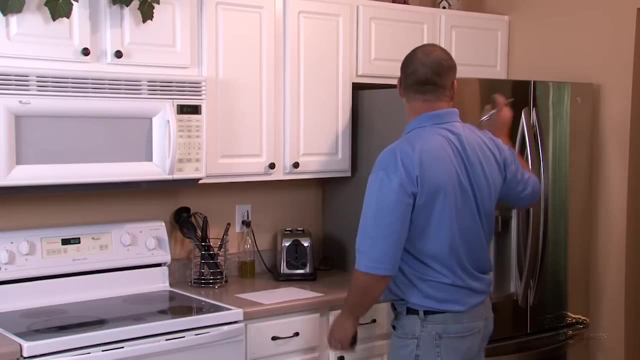 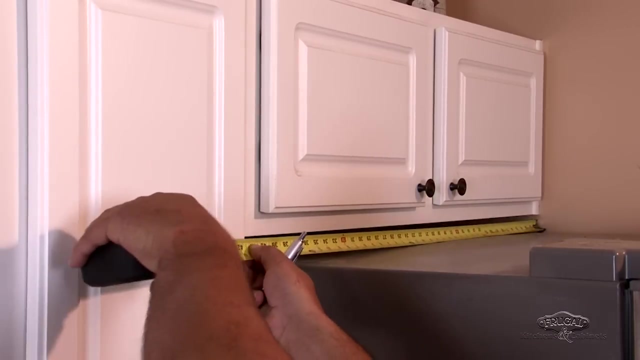 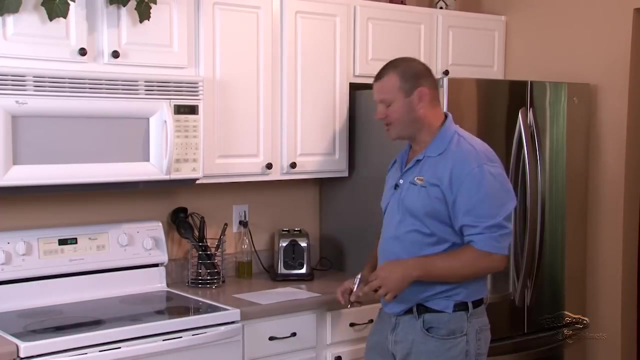 is the sink, So we'll draw the sink in. Okay, we're ready to start measuring, So grab your tape measure. You need to measure from the wall to the edge of this cabinet. Bring your tape measure over, Touch the wall, Measure over. We have 39 inches, So we're. 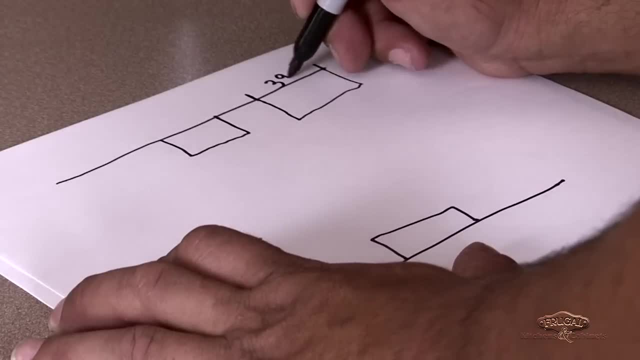 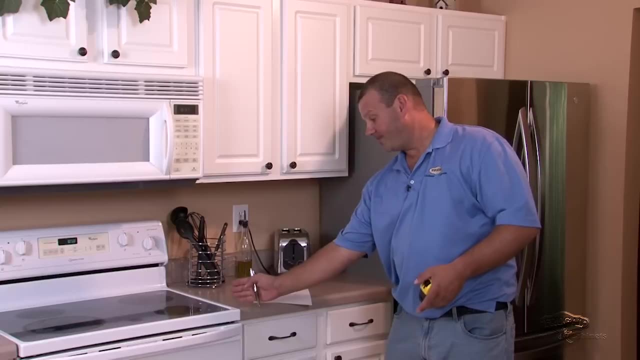 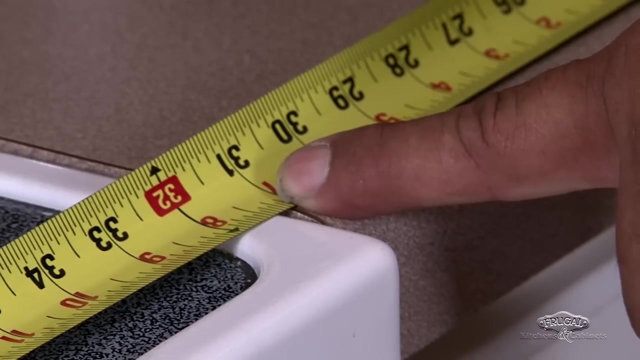 going to measure from the wall to the edge of the countertop, to the edge of the stove, 39 inches. Now we need to measure the space here. So from the edge of this countertop to the edge of the stove, replace the tape measure here over here: 31 inches Next. 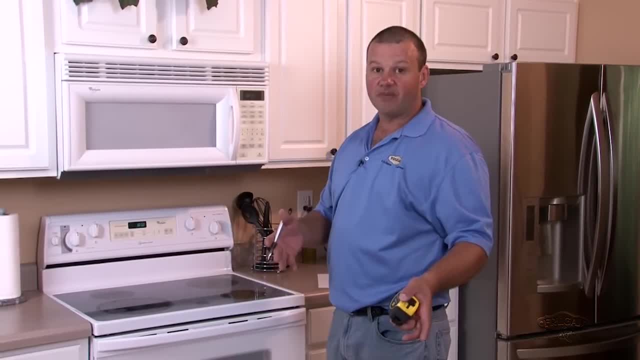 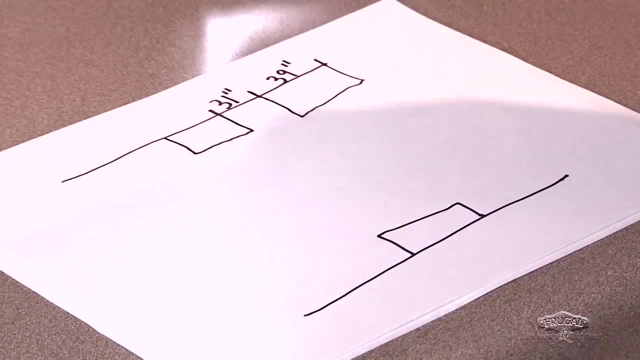 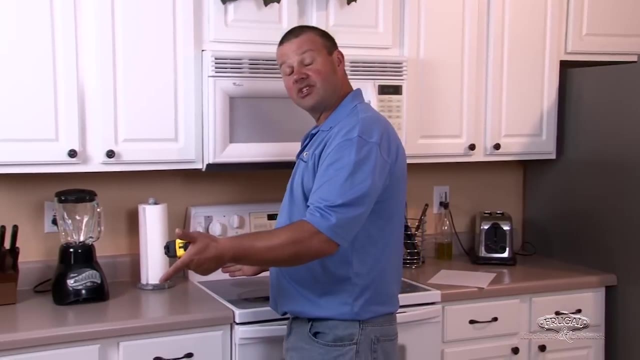 we have a stove. Most stoves are generally 30 inches, But for me I would double check the measurements just to make sure, Which means my turn marks were eliminated In this. sure It is 30 inches. Next we have a section of countertop, here again next to the stove, That is. 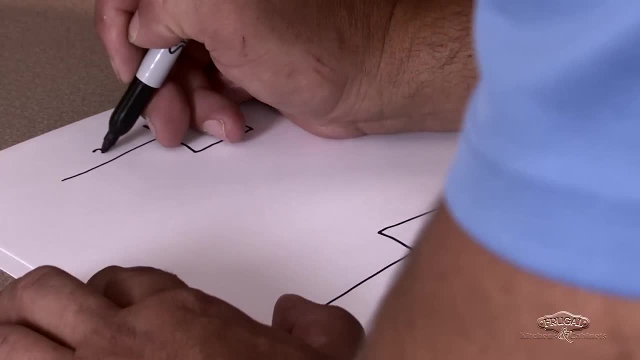 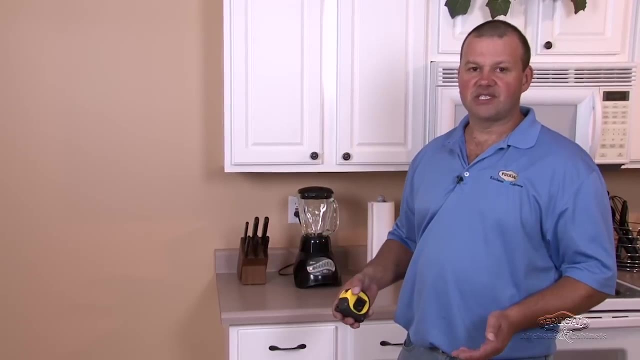 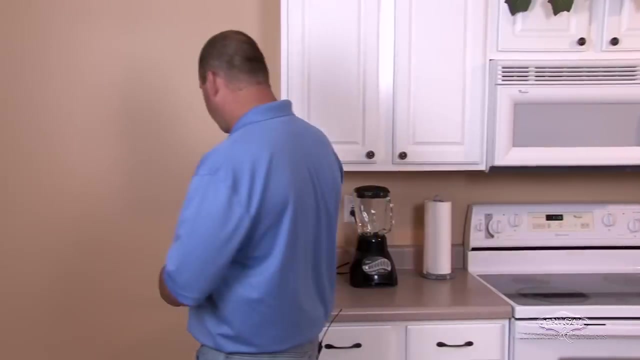 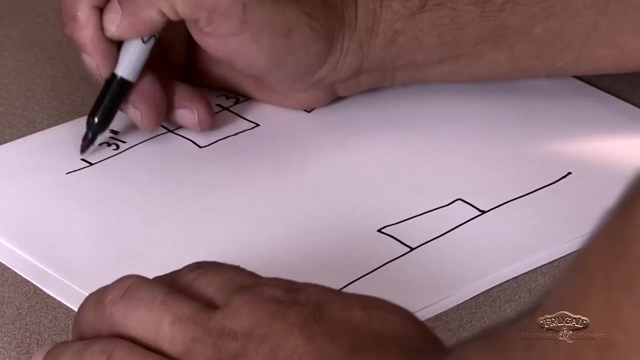 also 31 inches. Okay, that would normally be the end of this wall, but this customer would really like to have some more cabinet space, so we notice that we have some extra wall here. We've decided to come over and measure from this corner over 18 inches, and they can get 18 more inches of cabinet. 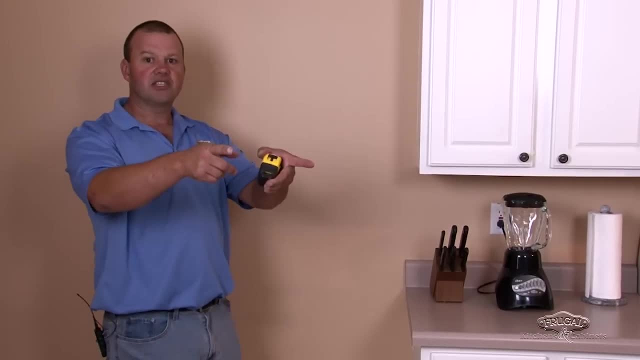 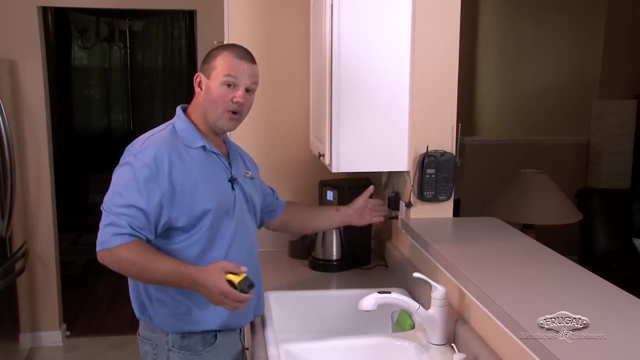 Okay, now that we have this side of the kitchen done, let's go over to the sink wall. Okay, the last thing that we need to do is measure this section of cabinets. All right, we need to get the overall dimension first, So we go from that. 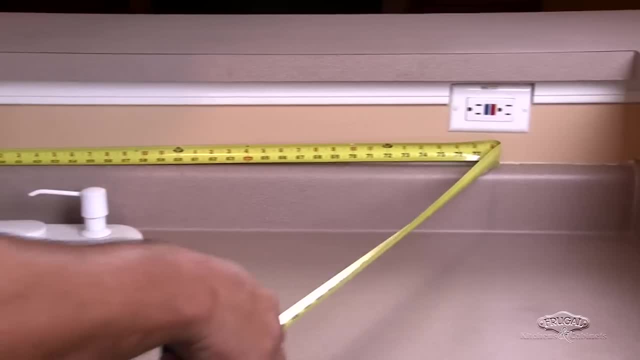 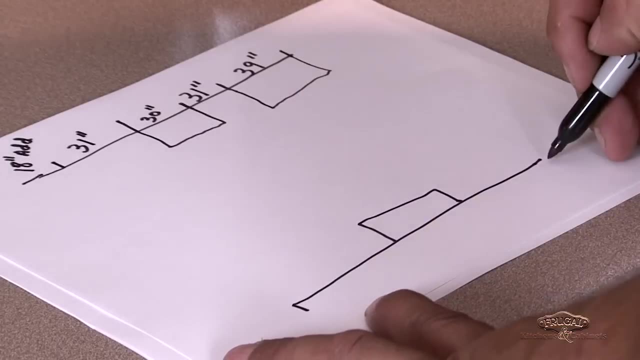 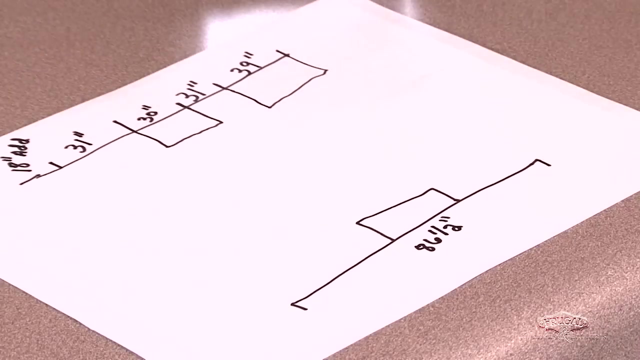 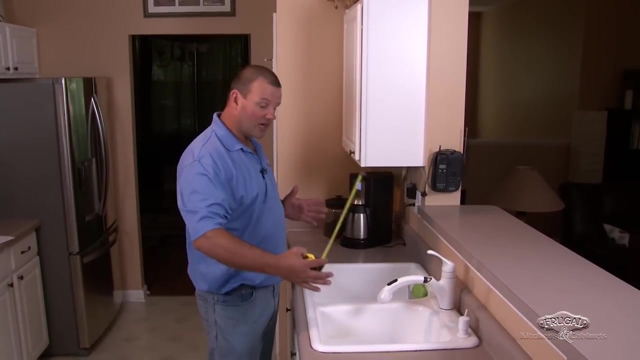 corner of the wall 86 and a half inches, We have this small section of wall 27 inches. Now we like to get the wall to the center of the sink. That way there I know how much we can move the sink left or right if we need the space.